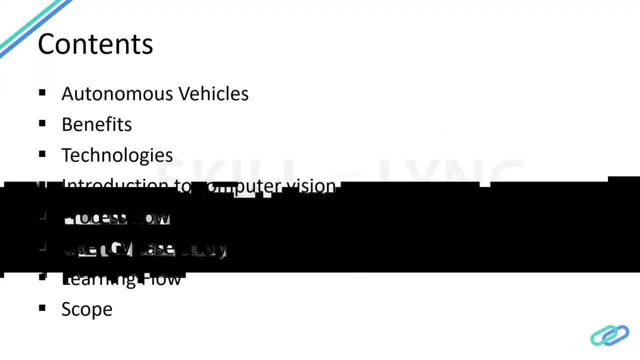 on the same page with what is an autonomous vehicle and how can we see an autonomous vehicle and understand the benefits of an autonomous vehicle, which, when an autonomous vehicle comes into road, what are the benefits that we're going to be seeing and benefits that we may already know? 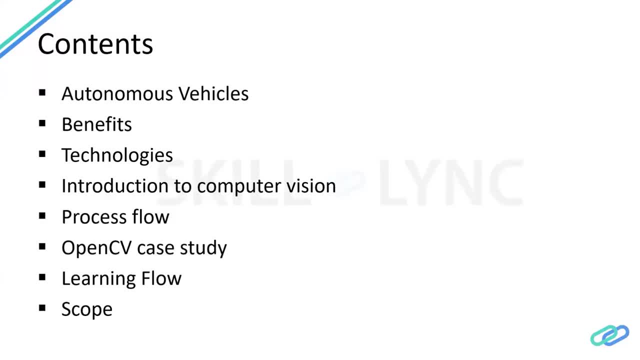 or we could already guess- and benefits that we may not know. We will be touching them a bit and the technologies that enable an autonomous vehicle. From there on we would be getting into computer vision. What is computer vision and what is the process flow for computer vision? 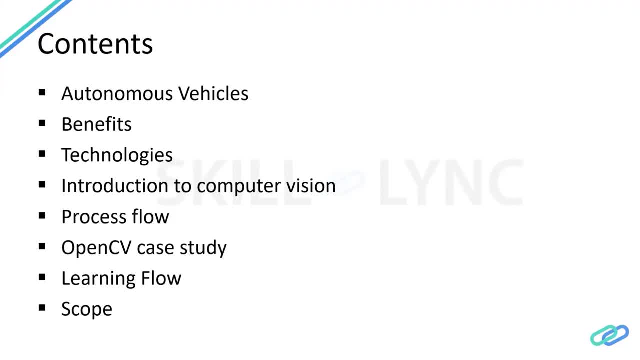 So there we're going to be talking about. what is the generic process flow right from the first stage in the computer vision to delivering the output for a specific task. What are the processes involved in between? and we're going to be doing a small open CV case study. I shall introduce you. 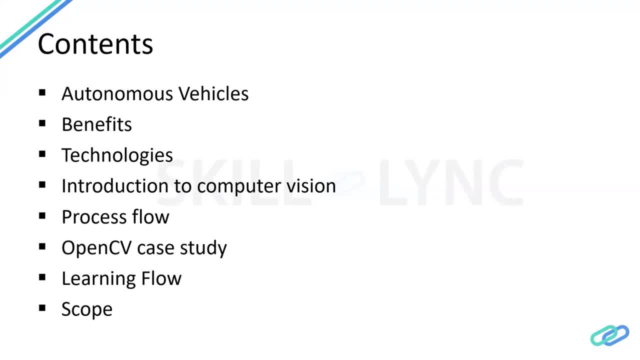 to open study. for those of you who don't know what that is and how we can use open CV for that particular task, So that is what we are going to be talking about in a little bit. So the open CV is a case study that is going to be done between there in the industry supporting 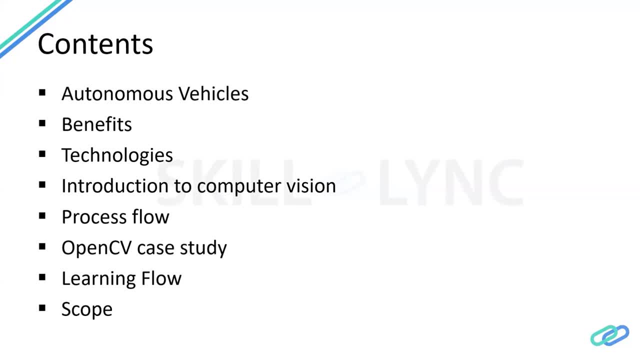 majority of the computer vision engineers, And we are also going to be seeing a case study which where we're going to be seeing an application where the open CV libraries would be used to solve a real world problem in autonomous vehicles. So that's going to be fun Moving. 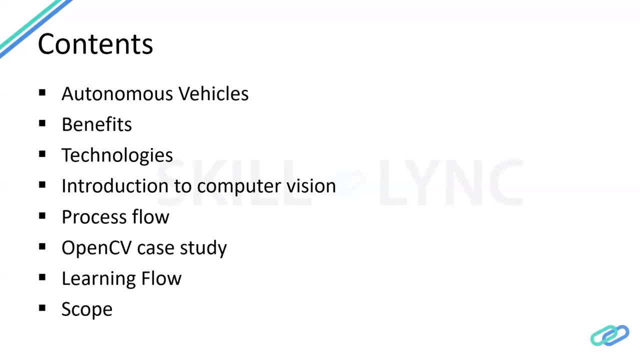 on. we are also going to be speaking about how you can become a computer vision engineer, What are the requirements and what are the topics that you need to know to become a computer vision engineer And, last but not the least, are we going to be speaking about the scope. 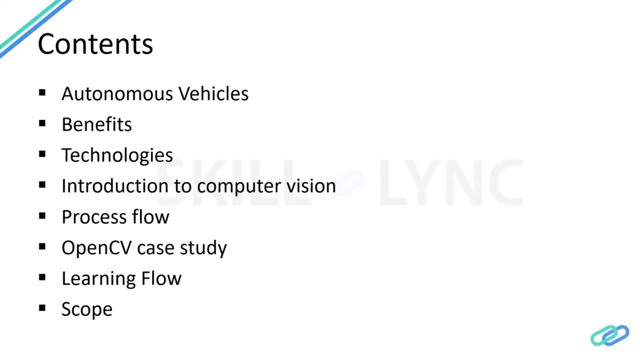 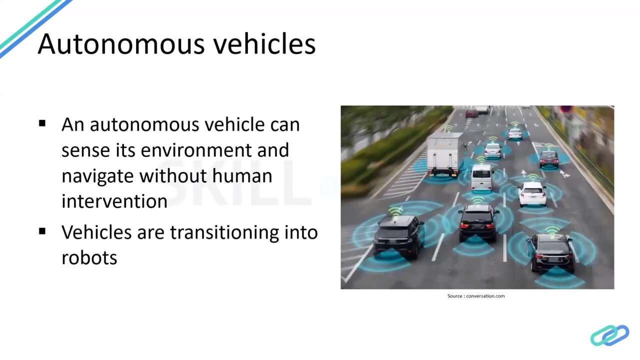 of a computer vision engineer in the current industry. What would a computer vision engineer do, and what are industries could he or she be applying to? We're going to be walking through all these topics in today's webinar. To start with an autonomous vehicles. we're 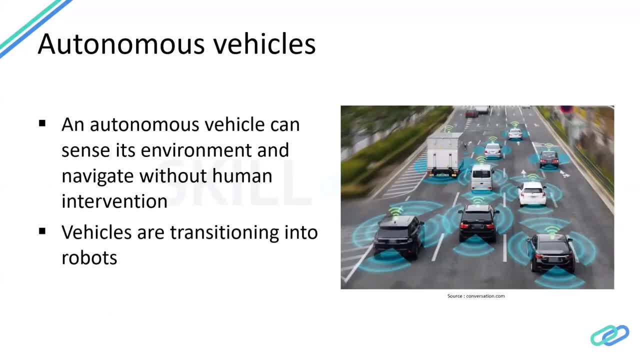 going to be talking about the scope of a computer vision engineer. So let's start with the scope of a computer vision engineer. So what is an autonomous vehicle? An autonomous vehicle is essentially a vehicle without a driver. Imagine it like this: You don't have 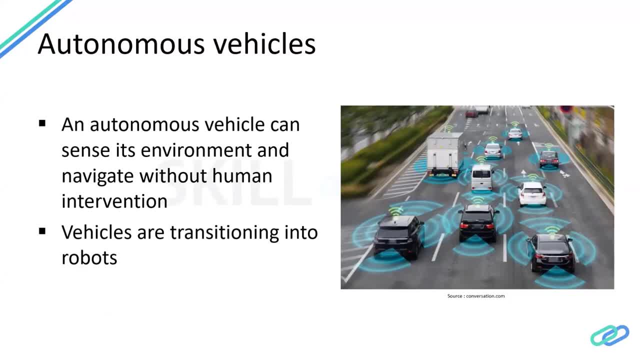 your steering wheel, you don't have your brake accelerator or any system that a driver uses. And imagine you having a dining table inside the computer or a work table inside a computer. And imagine a space like that that can move. Or, to put it another way, a train You're going. 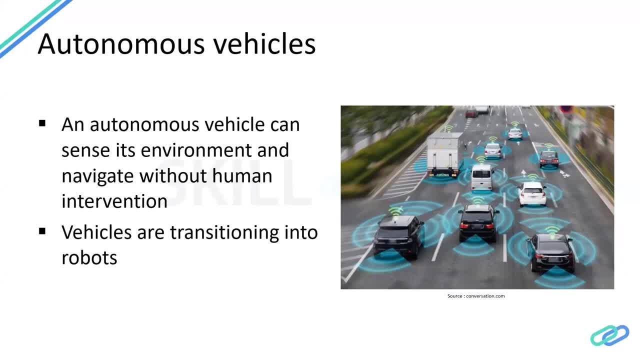 to be sitting in a train with the seats facing each other, and then it just moves, and without any intervention, it just moves by itself. So autonomous vehicles are essentially viewed as robots which can sense the environment, which can take decisions, and it can also aid the human being. 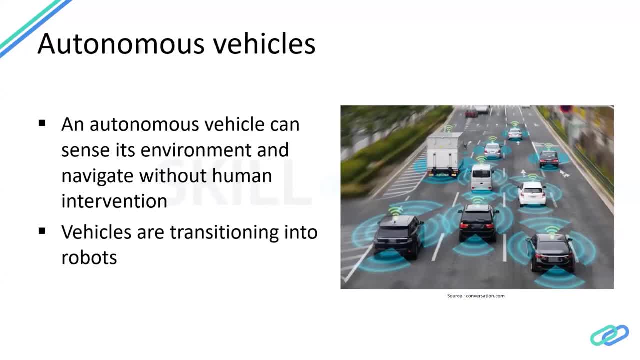 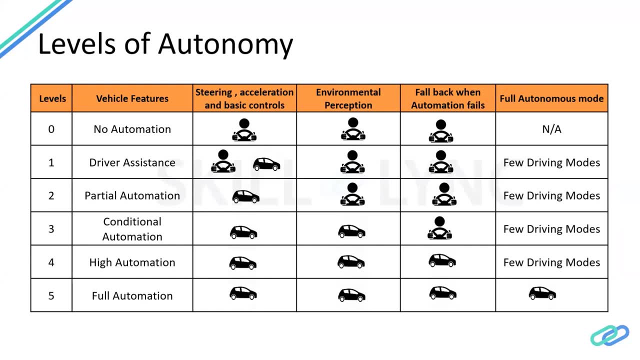 So autonomous vehicles can be used in other ways: while you are in the vehicle and also while you're outside the vehicle. Autonomous vehicles: the concept of autonomous vehicles, vehicles being self-driven- there's no necessary for a driver, and a consensus was reached around 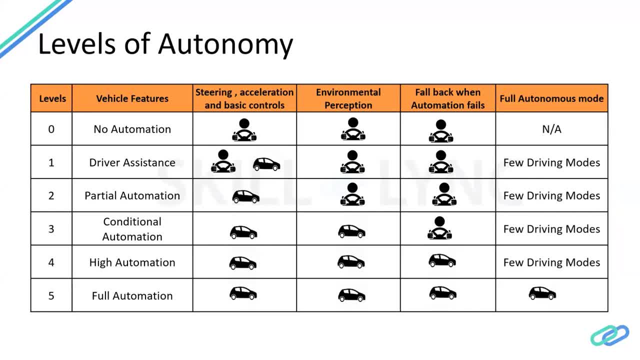 a decade ago on this that yes, we can. we should be moving ahead with this. A lot of companies started showing a huge amount of interest in this and engineers and researchers in SAE put together six levels of autonomous way Automation in autonomous vehicles. 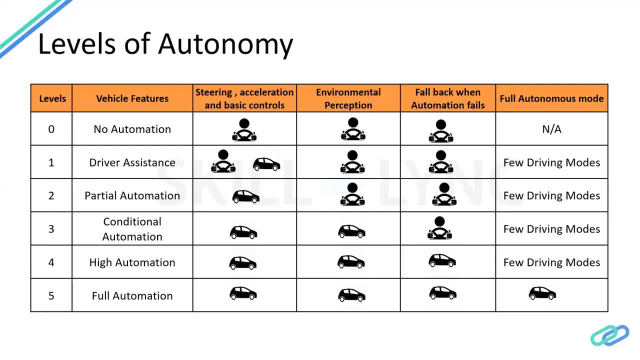 So we are, say, at the very least, the level zero, where there's no automation, everything has to be done by the driver. and then the other end of the spectrum is full automation, where everything is done by the vehicle by itself. And in between these two, as you can, 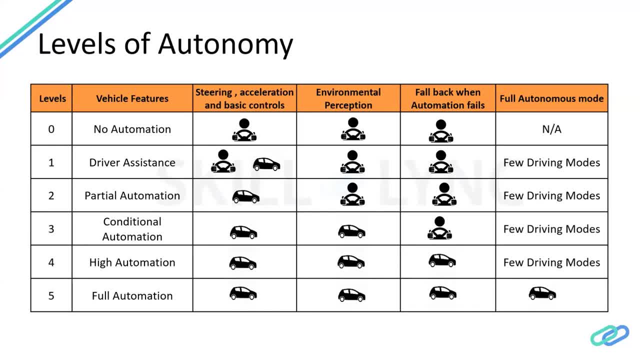 see on the presentation. you have two icons here, So one is the icon of a driver. So this indicates that for this particular vehicle, This particular action which is here in this case- steering, acceleration and basic controls- a driver would be giving his or her input And on the other end of the spectrum, 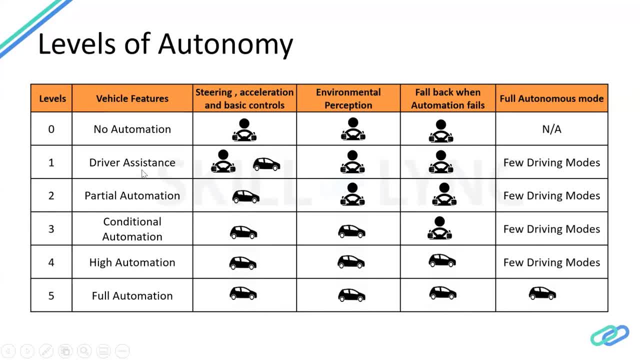 is a full automation where everything is taken by the car. Currently we are somewhere in between level two and three, between partial automation and level two automation. Some examples of partial automation, where the vehicle takes control of steering, acceleration and basic controls, would be features like lane keep assist. 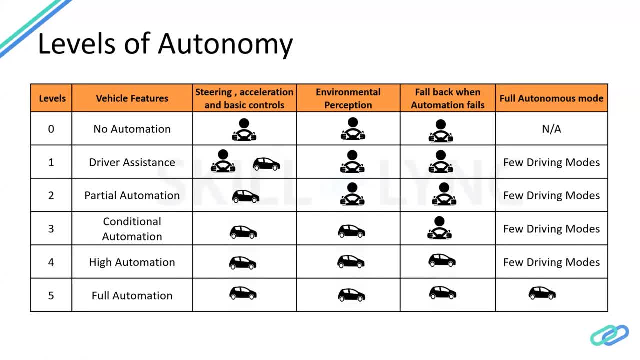 Adaptive cruise control, emergency braking, a few traction controls, So these things where the vehicle decides for yourself, based on what it can sense in the environment. Those features could come under the steering, acceleration and basic control features. And then the environmental perception is some. as of today, Tesla has autopilot out there which can sense the environment. 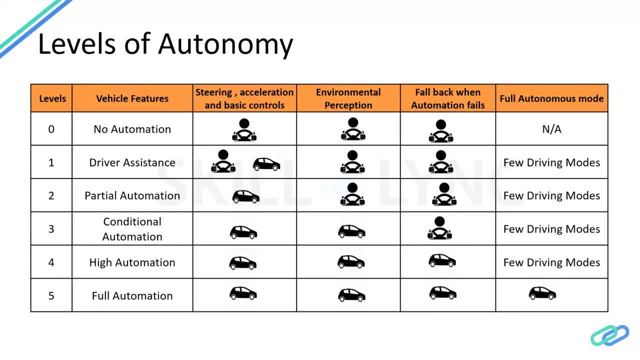 which can see for the vehicles, which can take decisions like shifting lanes, taking an exit in the freeway, which in Indian version would be like a highway, where you would be taking the service lane and trying to get out from the highway into the city. So these 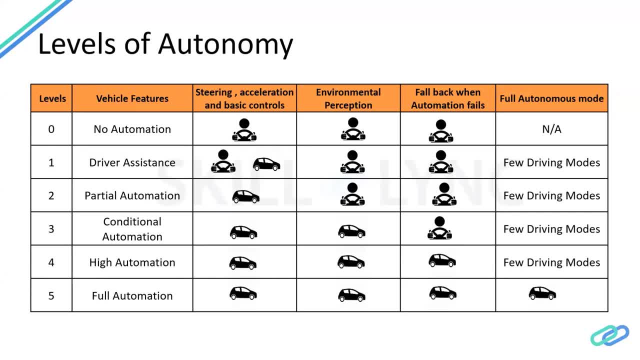 kinds of decisions are also, in addition, taken, So for which you essentially need environmental perception, which means that you need to know what's around you and where you are, and how you have to be navigating through the environment. Yeah, thank you, So I think that's a great question. I think that's a great question. 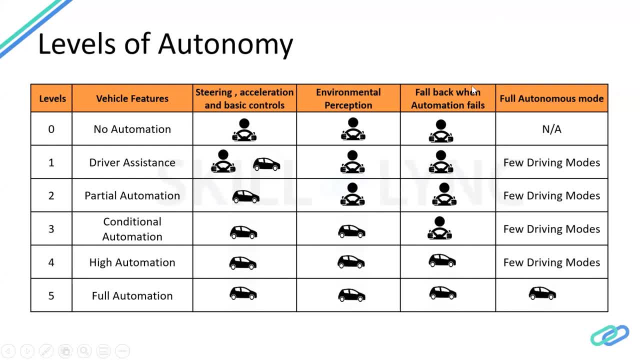 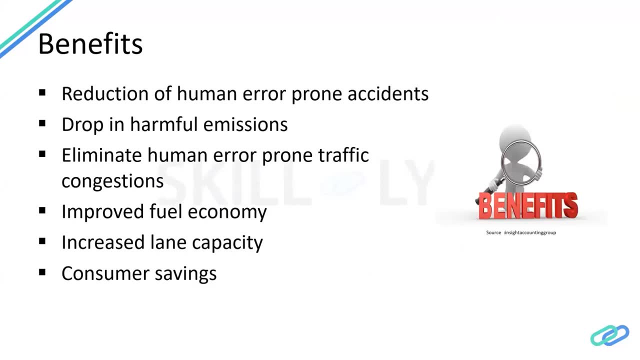 environment given to you, yeah. how you would be navigating the environment given to you, yeah, uh. and moving from point a to point b based on the objective. so moving on to the next slide, uh, the benefits of autonomous vehicles are: reduction of human error prone accidents. so most of the accidents, like, in fact, 95 or maybe even more the accidents, are due to human error. 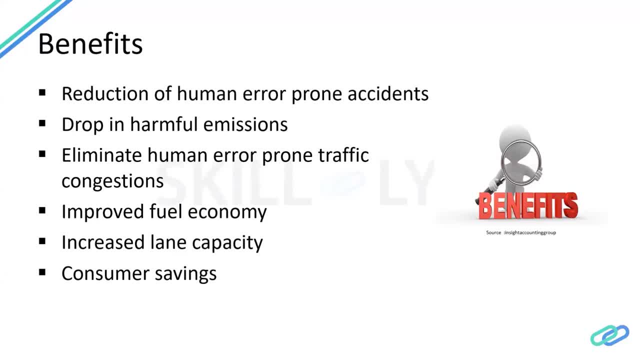 we are human beings. we are born to error, whether it's your error or whether it's the other person who's who who's driving the vehicle is going to collide into your vehicle. uh, most of the accidents are due to human error. uh, drop in harmful emissions. so here, uh, there are multiple. 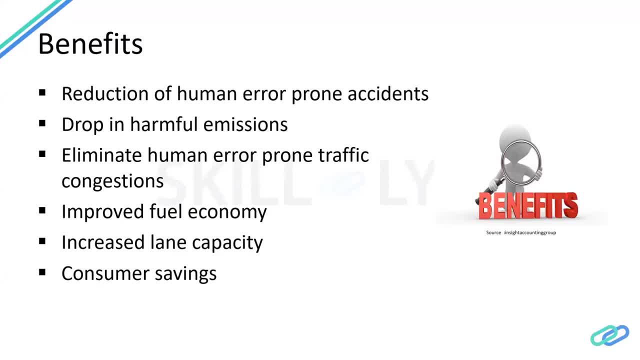 ways. uh, an ideal driving behavior on road would lead to the least amount of emission that the vehicle can give. so, based on your driving behavior, based based on how you rev up the vehicle or based on how you control the vehicle, the emission levels is going to change. so once you hand over the control. 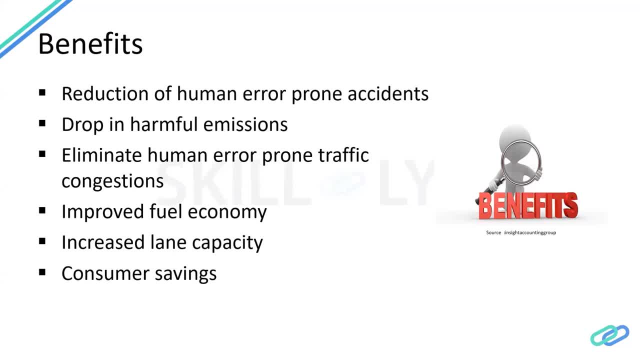 to a machine, it's going to take care of the best possible emission and uh, yeah, there's going to be a significant drop in uh emission and with the current trend of vehicles moving towards uh electric vehicles- and there's- there's definitely going to be a drop that way as well. 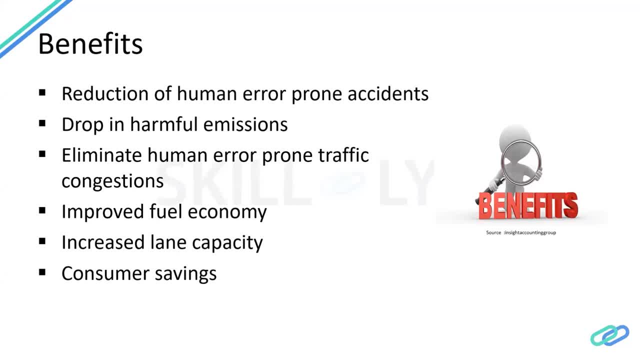 and eliminate human error prone uh traffic conditions. majority of the traffic conditions that we see on road is due to human error, like somebody wants to take a shift in the lane, somebody is is suddenly slowing down for no reason, or somebody, uh is seeing something very interesting on the road and wants to slow down. 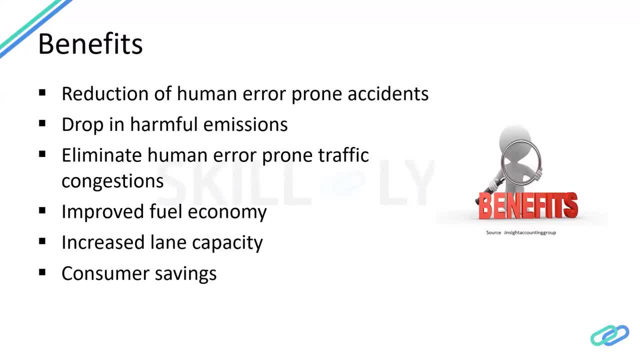 just so that he or she can take a better look at it. so these things uh lead to traffic conditions which, uh, we may not really see it firsthand, but then these things add up and then, which would result in a huge traffic condition, so an improved fuel economy, as i said earlier. 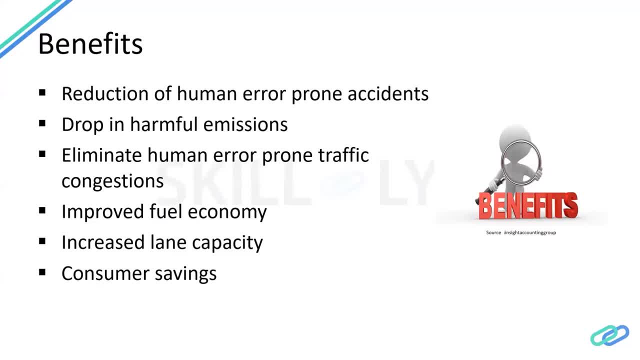 about emissions. uh an an ideal driving behavior? can lean also lead to the optimized fuel consumption, where you wouldn't be really spending as much fuel as you would when a human driver drives in an erratic fashion, where the driving uh style consumes more fuel and then uh increased lane capacity. so 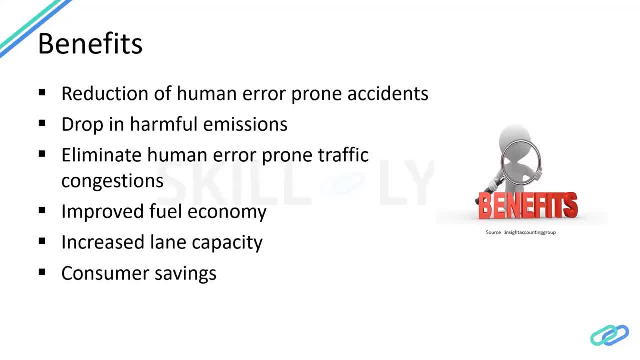 this is. this is another very important thing because, uh, right now, we tend to maintain a gap of- so, at least here in the united states- uh, we tend to maintain a gap of about easy 10 meters between, yeah, one vehicle and the other, and, uh, that, that. 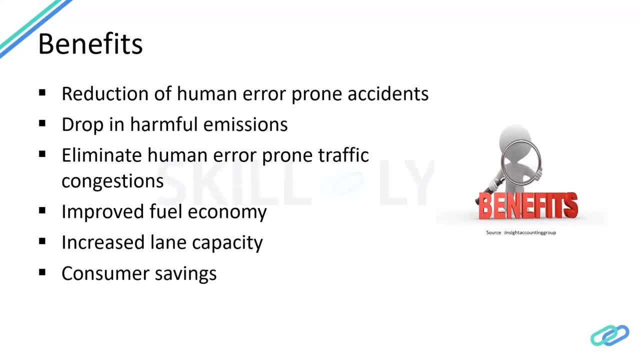 is so that you give some space for uh, the other human driver, to make an arrow. if he or she suddenly breaks the car or uh wants to shift lane, you give the buffer space for such errors. and when, when a machine has taken control of the car and one mission can, 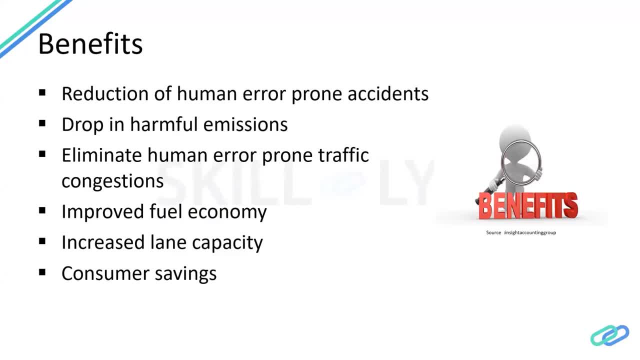 communicate with the other. this particular lane capacity can be increased by squeezing more cars in a limited space, by essentially reducing the space between one car and the other, and consumer savings, uh. so these things like things like fuel, increased lane capacity and one per like, multiple people using the same, uh same car, could all add up to savings in terms of. 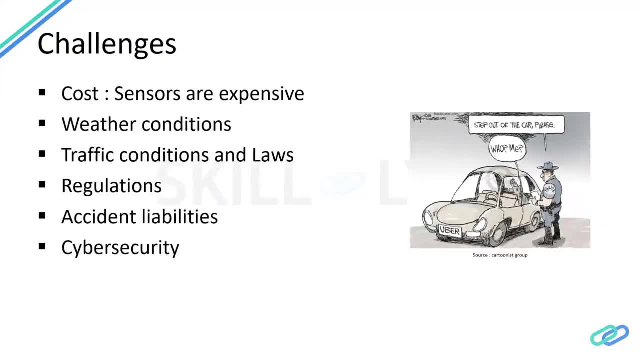 money uh to the consumer. so challenges are numerous in our autonomous vehicles. so, as we are still transitioning towards autonomous vehicles, vehicles, as i had mentioned earlier, are in essence, uh, robots. so robots would definitely require sensors to perceive the environment that you are in. and the sensors are complicated because 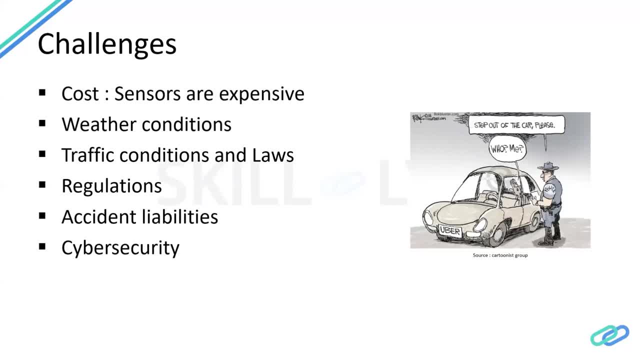 we human beings have evolved over thousands and thousands, probably even millions of years, to develop certain qualities that we we see and we perceive about our environment. so developing a machine that can mimic or probably even do it better than us, uh, would require a lot of sensors, that which are in turn, expensive, and also there are multiple things that adds on. 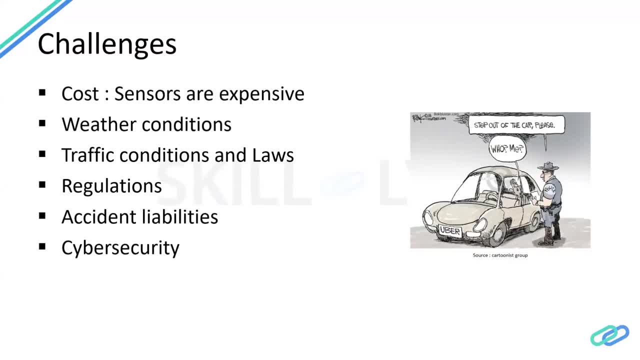 to the cost of the sensors. one of the thing, uh, one of the major place where a lot of cost is added are to the vehicle is the processor then, and second challenge would be the weather condition. so, um, even the human visibility are drops in times of fog and when there's rain and there's snow. 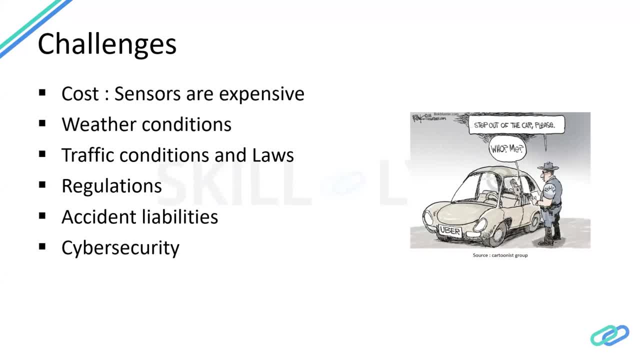 this could be another challenge, and for autonomous vehicles, the traffic conditions and laws could change from one place to another. for example, a car that is made to be driven around in the united states may not be readily applicable to indian roads, for example. over here people use stop signs and there are specific speed limits. in on the highway there's 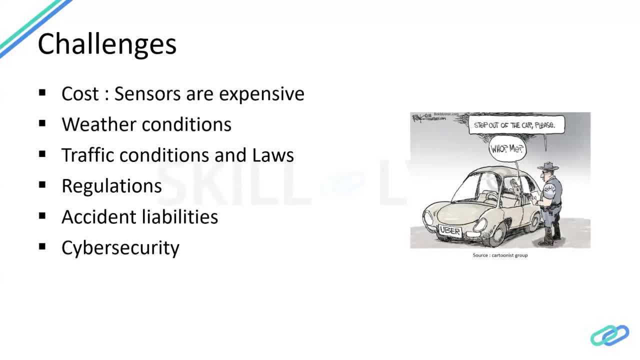 a lower speed limit as well. and then there's higher speed limit, which may not be really applicable to other countries, or a lot of uh, even in the case of tesla, the uh, the the traffic rules are very different between united states and europe, so uh, where a lot of custom models are. 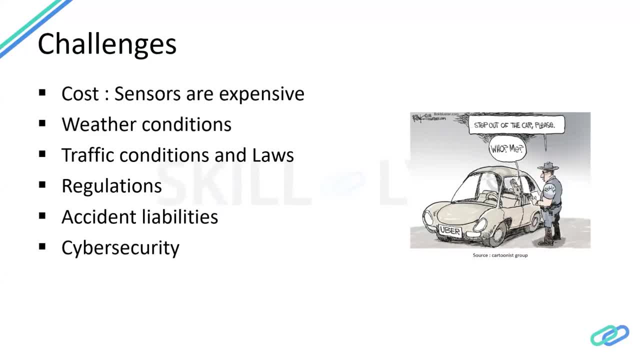 built that. can uh address those conditions? and then regulations. as you can see in the picture, it's a little funny, right? uh, the cop pulls over the car and then uh asks the person to step or driver to step one. there's no driver there and uh, so such accident liabilities and regulations. 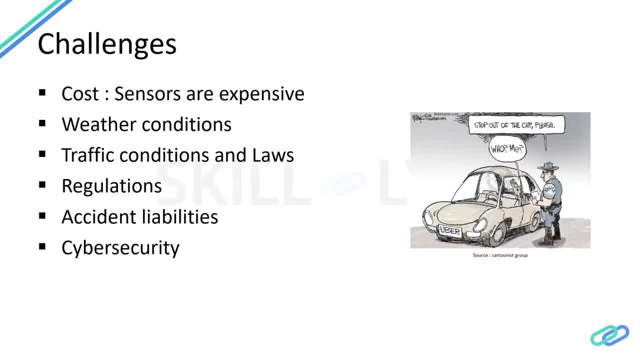 could also be a challenge that has to be addressed. uh, and i just want to layer on to the fact that, because of all the reasons that i told you, the way like the best way to counteract the issue and to change the way you think, you think. 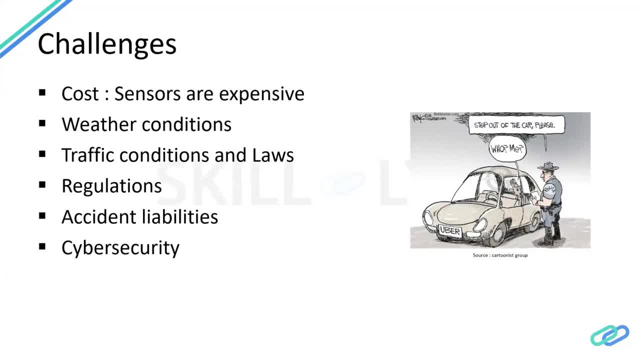 should be dealt with by your parents is in a very short term way, and we're in time for you. so the question is: which policy should we adopt and how should we do it? what the policy should we adopt should we do? what the policy should we do about it? and then i think it's a very important. 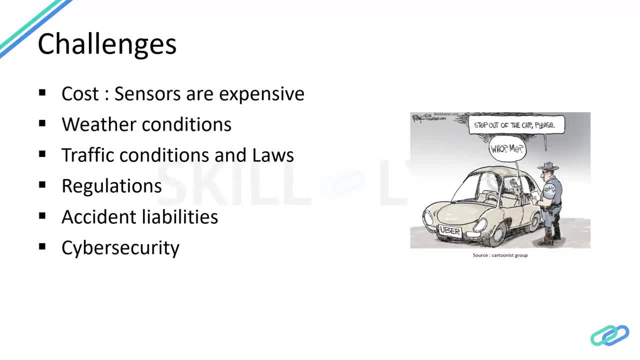 question right now that a lot of progress is being made in the future that we have to come to. Cybersecurity is another field where technology presents a challenge and it's also an obstacle to autonomous vehicles becoming a reality. So these are the areas that are being worked on and also, you know, obstacles that will be worked on in the future for the autonomous vehicles to become a reality. 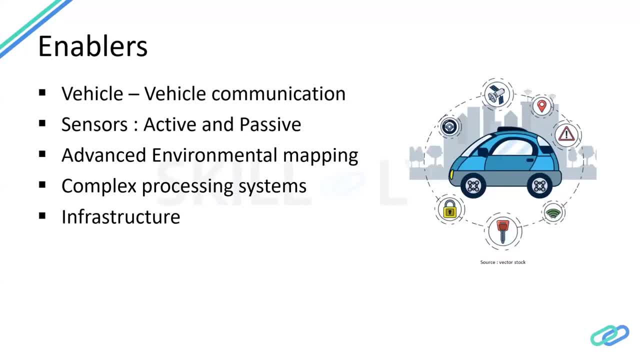 Now that we've seen the obstacles, what do we think are the enablers? By enablers, I mean things that enable the system to become an autonomous vehicle, enable the robot to navigate by itself. So one of the important concepts required is vehicle-to-vehicle communication. 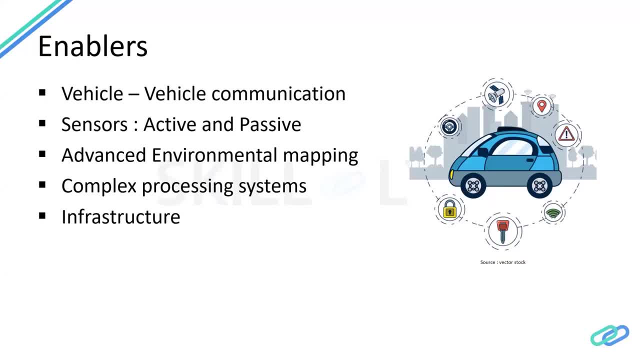 That is very important, given that all the vehicles are going to be robots and they ought to be communicating with each other to know where one is respective to the other and how change in one vehicle's path, So that would affect the other vehicles. So a good amount of communication and engagement is required between vehicles on the road so that they do not commit any mistake. 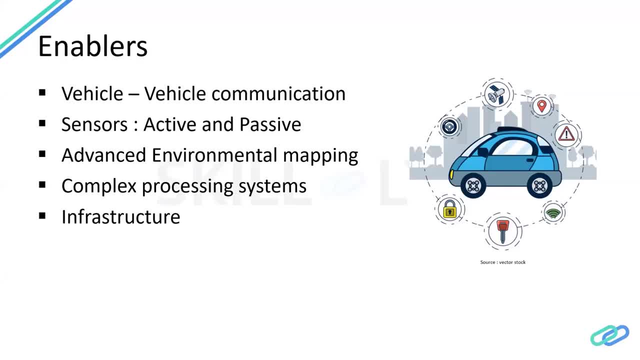 And sensors. active and passive sensors are both required to enable an autonomous vehicle, And by active sensors I mean sensors that are like cameras, and then by passive sensors. passive sensors can be anything that in turn, which are directly not involved in the vehicle. 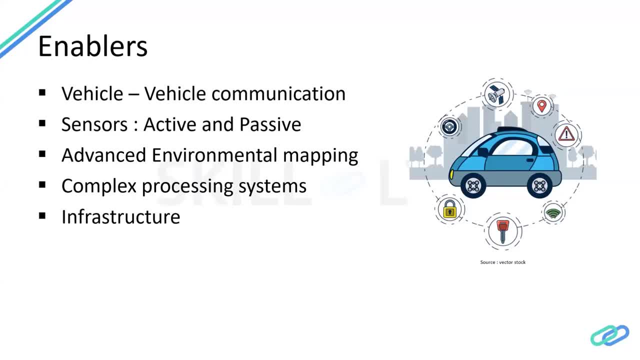 So that's one of the things that we're working on. So that's one of the things that we're working on, And advanced environment mapping is required. If you see today's GPS, many of us would have gone through this problem when we are using Google Maps, or any other maps for that matter. 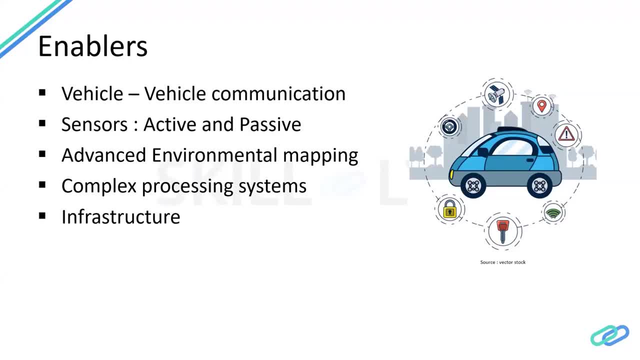 You would miss a turn easily, right Like you would miss a turn and map would take some. there would be a lag between you seeing the map and the map responding with the right route And then you would miss the turn And these kind of interventions. 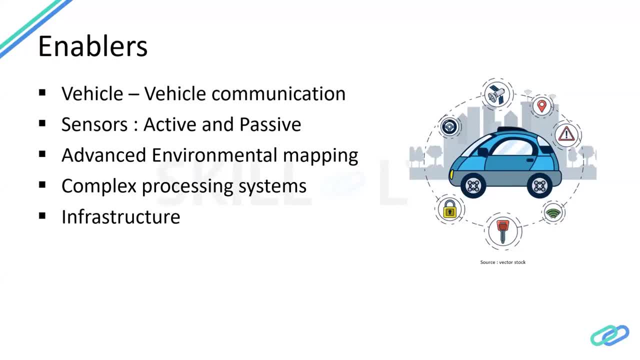 Inaccuracies cannot be there for a machine when a machine is navigating through. So there should be high precise mapping and a lot of accuracy. by that I mean like accuracy to the levels of few centimeters or meter is required for an autonomous vehicle to navigate. 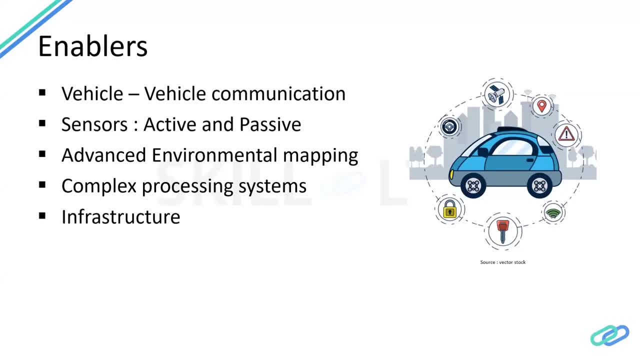 And complex processing systems. as I had already mentioned, processing systems can get really complex because the sensors that we're going to see- An idle camera- is going to give you Frames at 30 frames per second, which is a lot of information, given that every pixel takes at least eight bits. 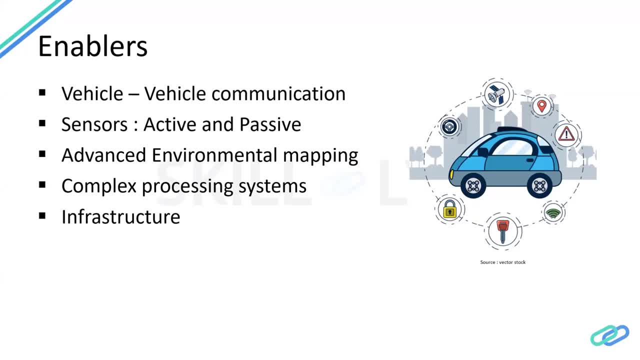 And then you have these high resolution cameras, which is going to pump in like millions of pixels at once, And then the processor should be able to process such an influx of information, which is going to be a lot, Given that you have cameras. you have other sensors, such as radar, lidars. 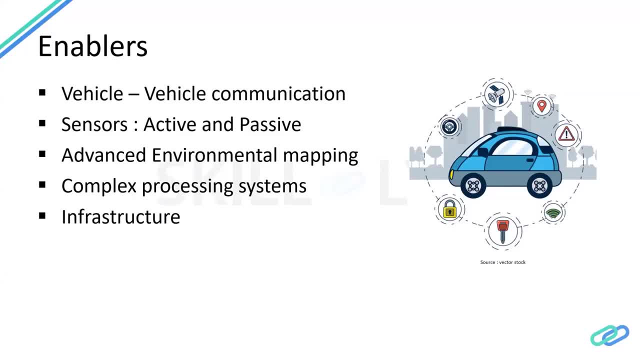 Then you have the sound Vibration Based sensors, and then ultrasonic sensors, And then you have many other sensors running In real time where it is very important for the processing system to be really quick in taking the decision, and then the infrastructure. 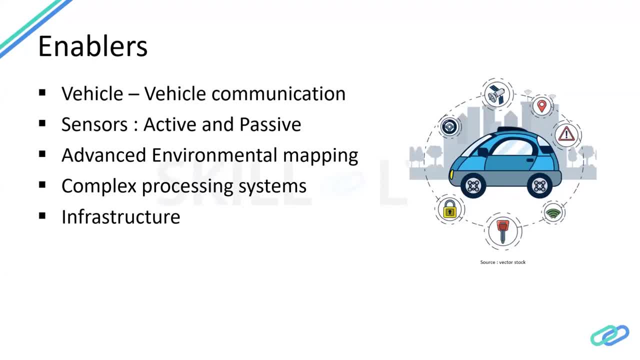 So for an autonomous vehicle, as you agreed upon, the vehicle is going to be like a robot, So robots need of specific infrastructure, a uniform infrastructure, to function. It shouldn't be surprised with Any alterations to the roads or anything that it has not seen before. 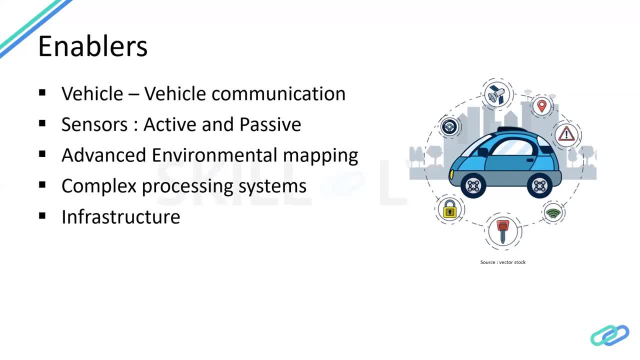 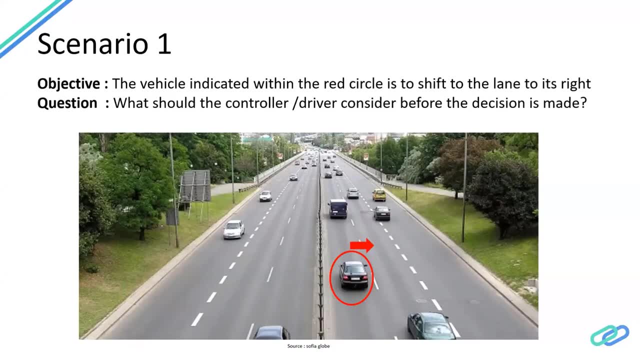 So an infrastructure is also required to enable such technology. The objective is, the vehicle shown in the red circle has to shift its lane from the current lane, which is the leftmost lane, to the to the middle lane Right. So the question is: what should the driver, or the controller as we call it, in the case of an autonomous vehicle? 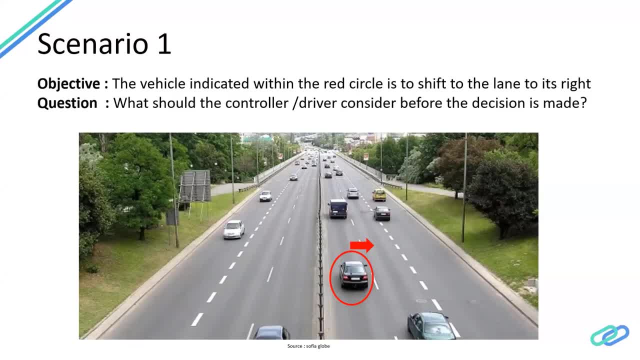 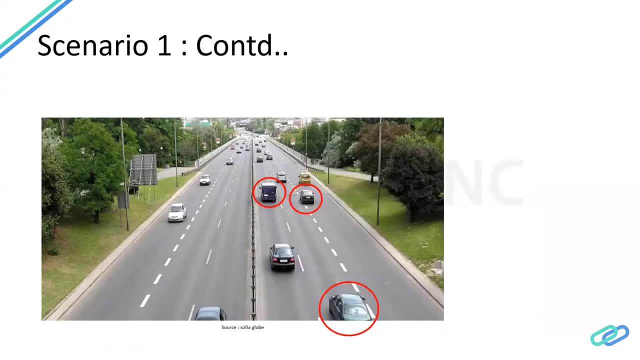 consider, before this decision is made, before moving from this particular lane towards the other lane, what all should it see? So, as we move on to the next slide, so we will see a few of the answers that I thought would be necessary. Those, though, these things do not cover a few of the answers that we just received from the participants. those are really valid answers. 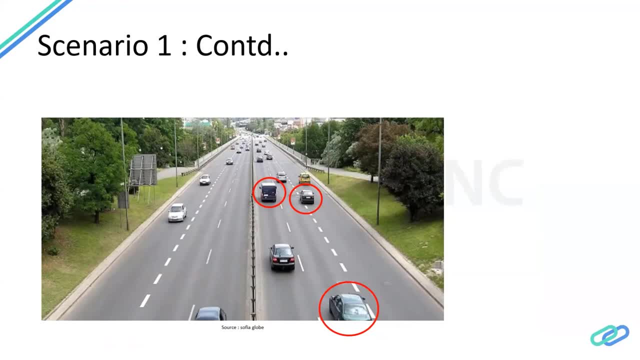 I did not add all the possibilities, which is very complex, So I have added a few. One is Object detection, because the vehicle has to detect what are the objects around it. As you see, there are like two cars ahead and then there's one car behind, as one of the answers that we got. 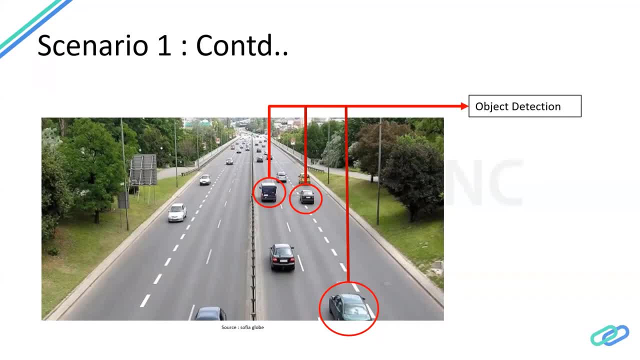 We should be mindful of the car behind and also ahead of us. And second thing is the object's parameters, vehicle acceleration and the path planning of the of of the cars. So when we, when we negotiate a turn, or when we, when we shift from one lane to another, as a human being, we do put some level of. 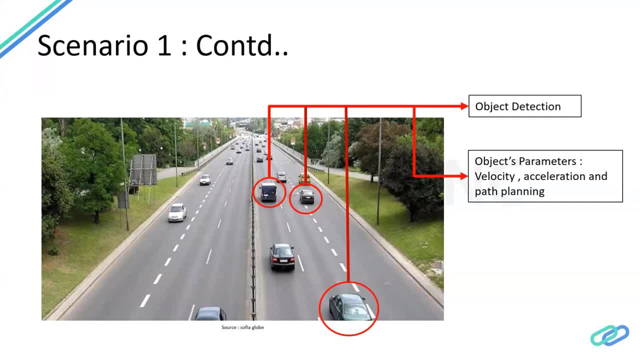 Trust on the other person, right, Okay, I'm going to turn now. This is: this person is not going to do something ridiculous that might end up being dangerous for me. So, when it comes to machines, that's where the vehicle to vehicle communication comes in place. 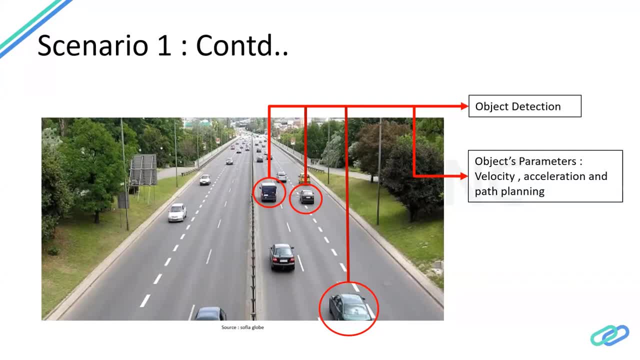 So if this particular car that we spoke about earlier, the black car that we see in the left, the leftmost lane, wants to change the lane, it would have to know what the other vehicles are up to right If the vehicle is going to cruise straight. 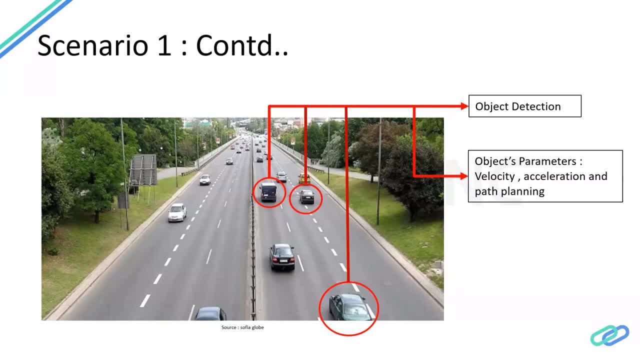 Through or like. imagine the vehicle behind it is communicating to the black. hey, I'm going to maintain a speed of 60 kilometer per hour And if, if you are going a little faster than me, you're, you're more than safe to, at least from my end, to make the lane switch. 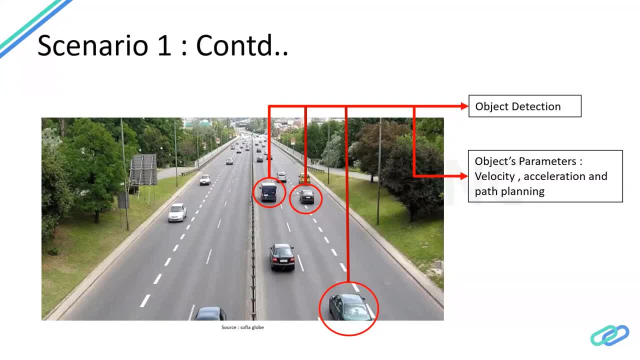 Now, that level of parameters are required, like velocity, acceleration and path planning of other vehicles and vehicle controls, is another Thing that an autonomous vehicle has to take care of, right like the its own vehicle controls, like steering change and acceleration, braking and whatnot. 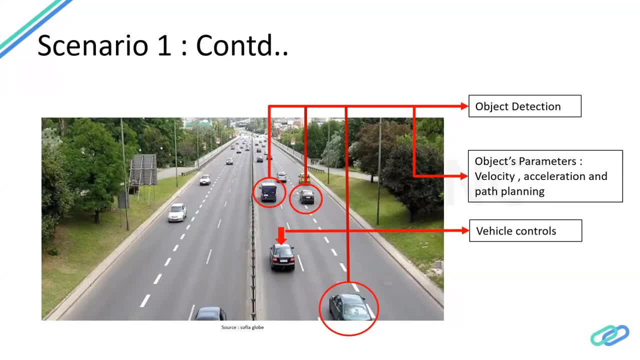 The indicator that somebody had mentioned. So these are the controls of the vehicle that an autonomous vehicle should be able to take care of. And then, yeah, it should. it should also run a check and be sure that it controls. it is in place to do that on, and self-positioning is very important. 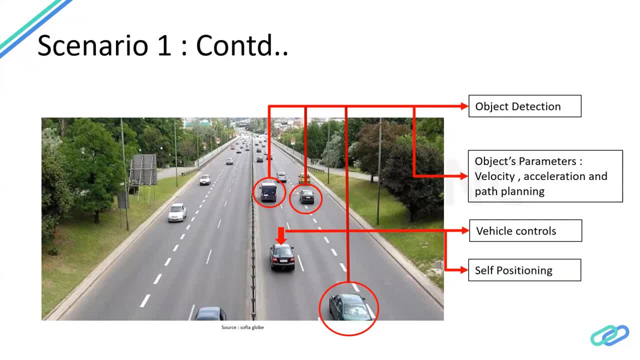 It should know Its position, say, in a global coordinate system or in a in a local coordinate system. it should be able to know its position with respect to other vehicle and also its own position, So that when it makes the turn it should know precisely where it's going to end up. and it should know its position every microsecond or even every nanosecond, where it is and where it's going to be in the next moment.